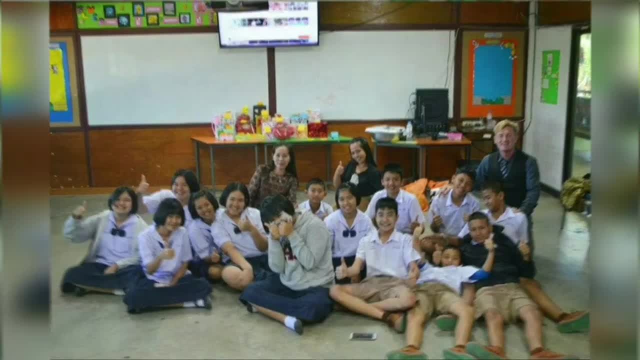 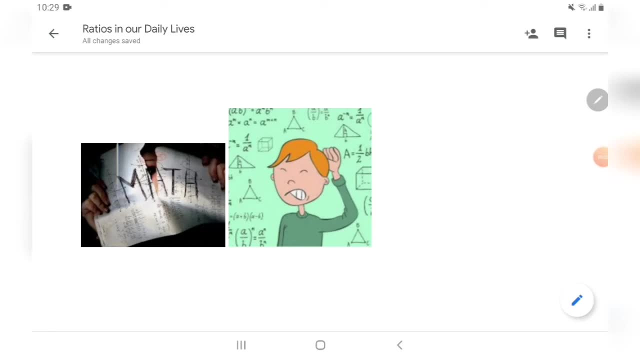 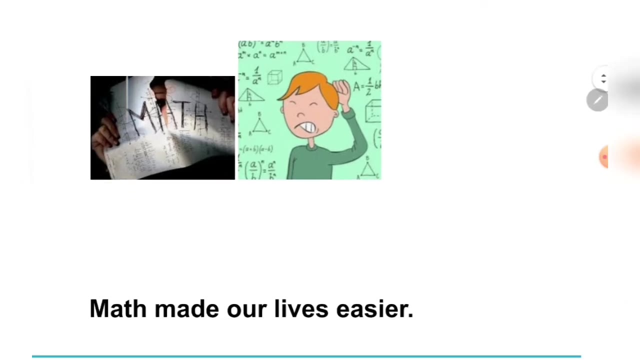 Thank you for watching. When we prepare food, when we manage money, when we decorate our home, when we do our gardening or landscaping like that, when we're figuring distance or time and a lot more, We don't realize that mathematics is everywhere. 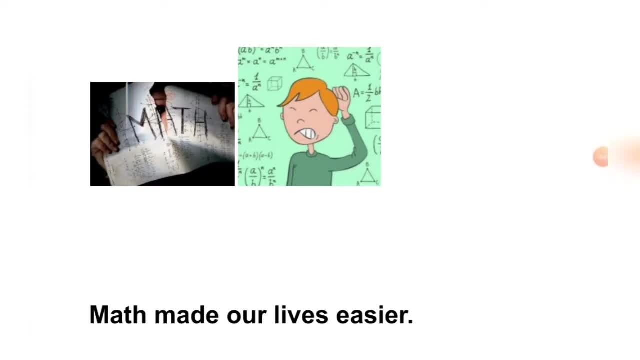 Also, math is applied to every profession. If you like to become a teacher, doctor or engineer, soldier, call center and a lot more- Every profession- you applied mathematics there. That's why, even if you like it or not, math is part of our lives. 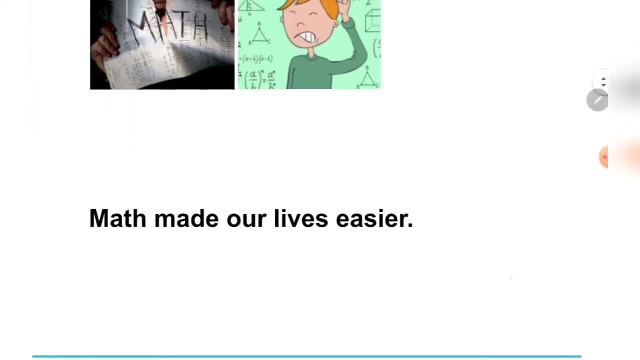 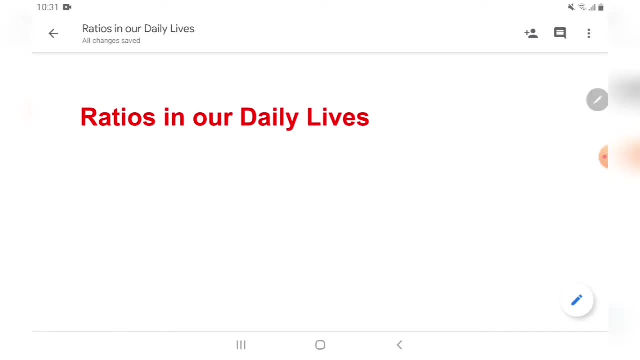 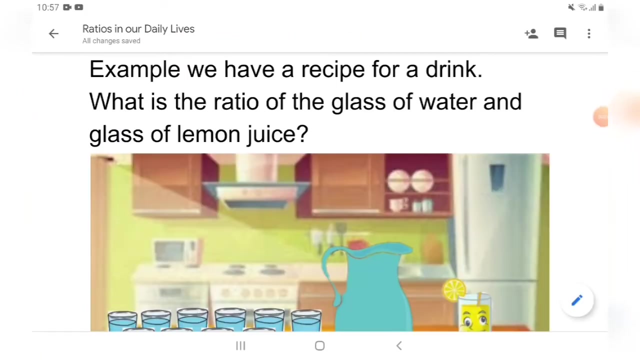 Because math made our lives easier. Even that math is difficult to understand, but it is. Math made our lives easier. Now, today we're going to talk about how can we use ratio in our daily lives. For example, we have a recipe for a drink here. 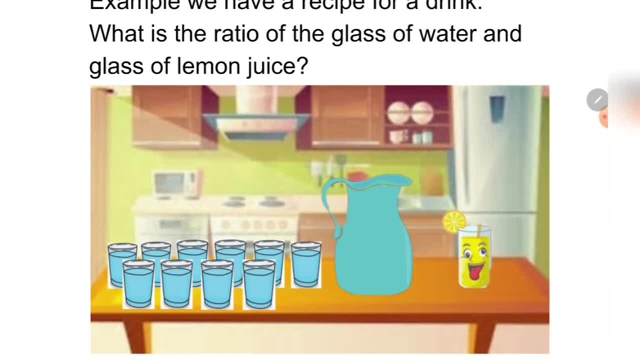 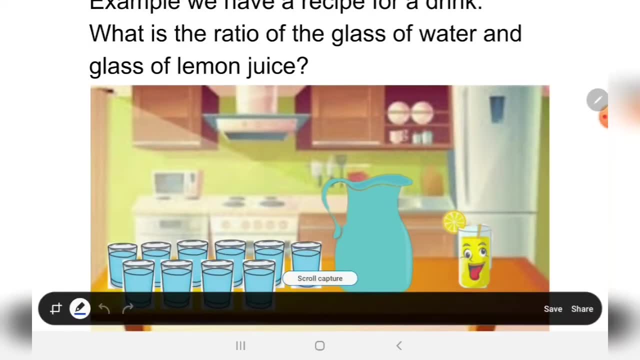 Now, to make a good lemon drink, we need how many glasses of water? That is 1,, 2,, 3,, 4,, 5,, 6,, 7,, 8,, 9,, 10.. So there are 10 glasses of water. 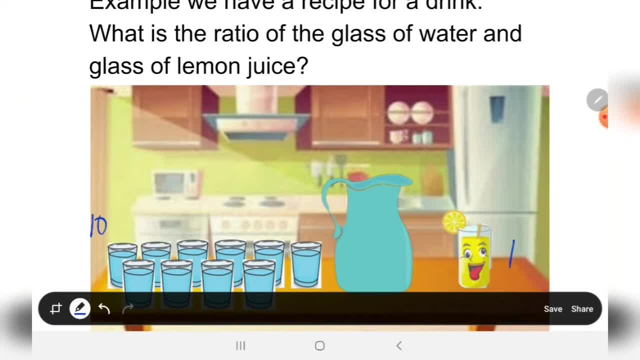 And then here is one lemon drink. So the question here, the problem here, is that we're going to find the ratio of the glass of water and the glass of lemon juice. We know that in here there are 10 glasses of water. 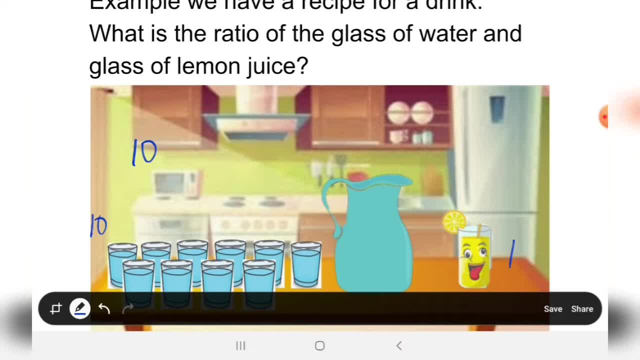 And then to make a ratio, we use the same Symbol, colon, and how many lemon juice and glass of lemon juice, and that is 1.. So the answer to our question- what is the ratio of the glass of water and the glass of lemon juice- is 10 to 1.. 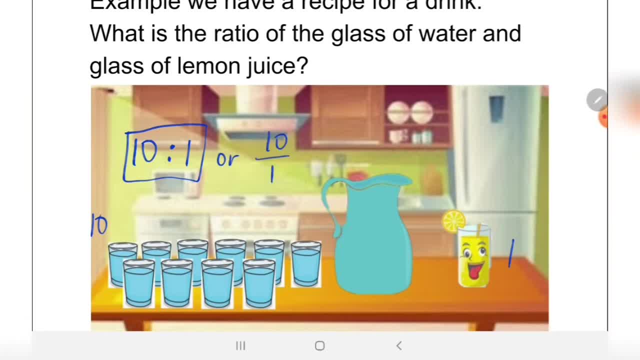 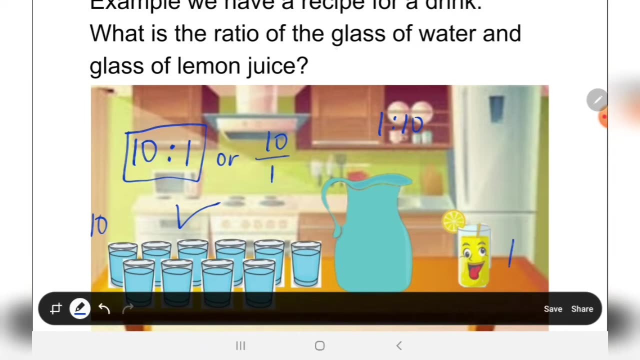 Or we can write that as 10 over 1.. Okay, So this is a good drink. How about if we reverse it Like 1, 2. 10.. What does it mean? It means that in here, since this is the first quantity, so this is 1 glass of water. 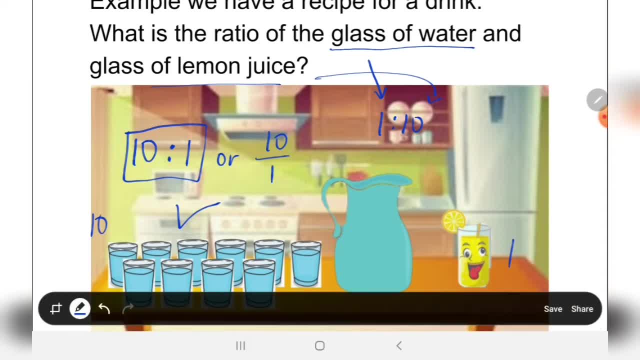 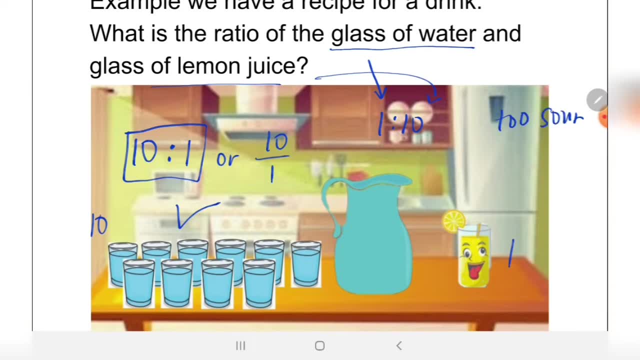 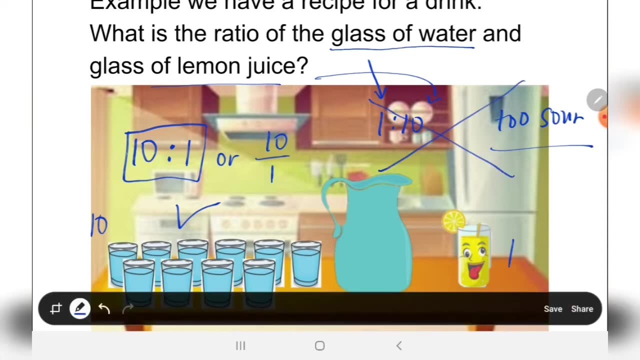 And in here there are 10 lemon juice. So what happened in our drink? It's too sour, It makes our drink too sour, So this is wrong. Okay, This is the correct Or the right answer. Remember that when we make ratio, we should follow what would be the first quantity and the second quantity. 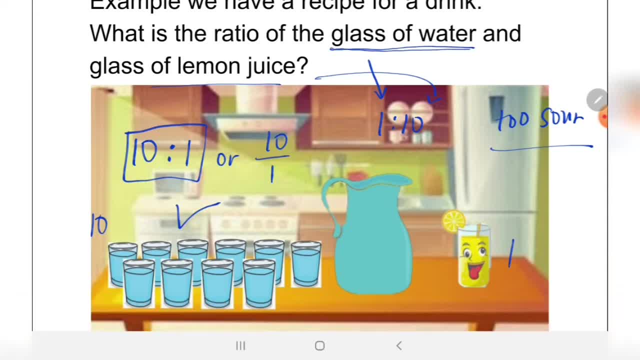 Remember, For example, in here the first quantity is the glass of water. So meaning you will count how many glasses of water in here, That is 10.. And here the glass of lemon juice, That is 1.. 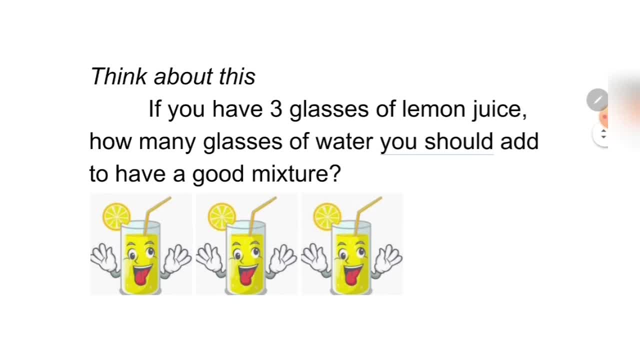 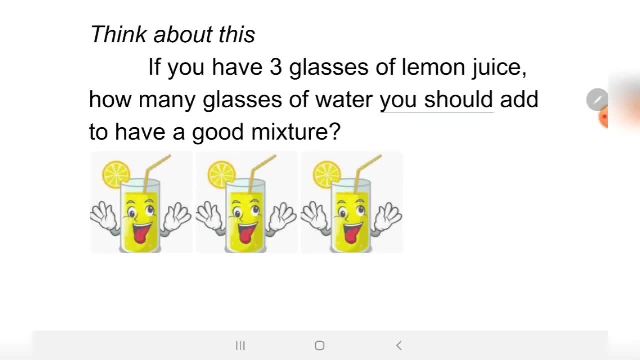 Okay, Next Think about this: If you have 3 glasses of lemon juice, how many glasses of water you should add to have a good mixture? Earlier we discussed that in every 10 glasses of water we need 1 lemon juice. 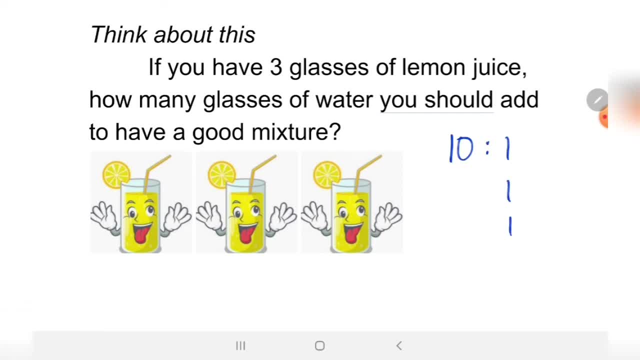 So in here we have 3 lemon juice And what would be, or how many glasses of water we need To have a good drink And that would be very good. That is 30 glasses of water. So in here, 10 plus 10, that is 30.. 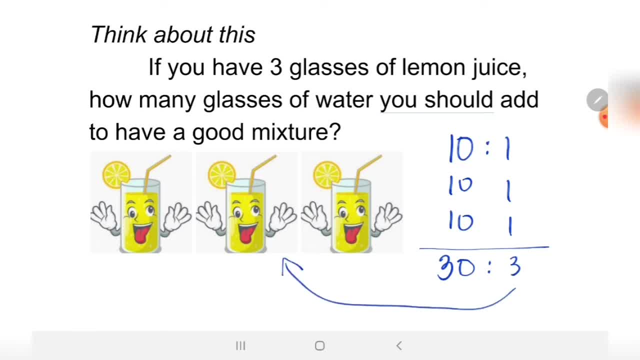 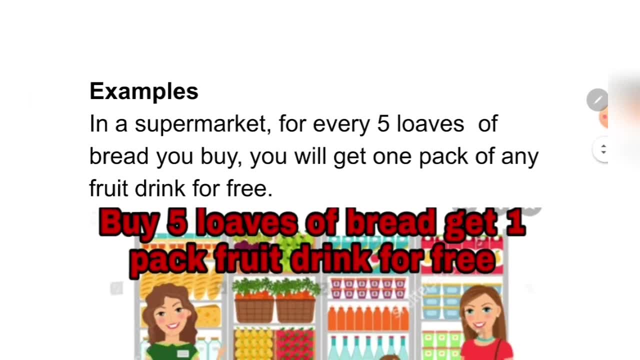 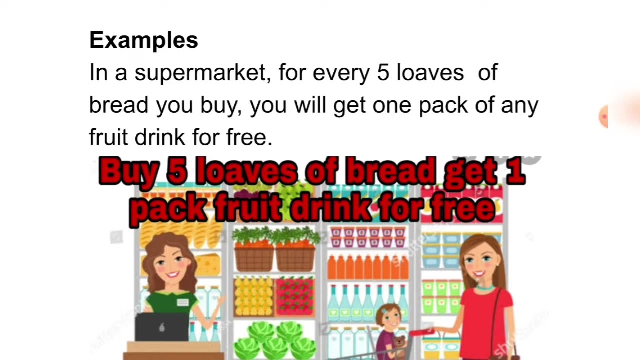 And there are 3 lemon juice, Remember. So that's answer to our question. Next, For example in here: Remember When you are in a supermarket And then There is a promotion there That for every 5 loaves of bread you buy, 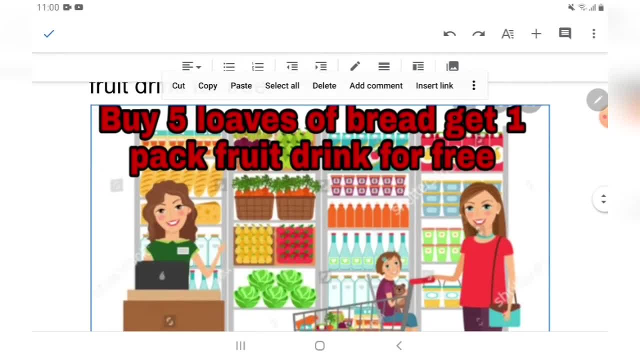 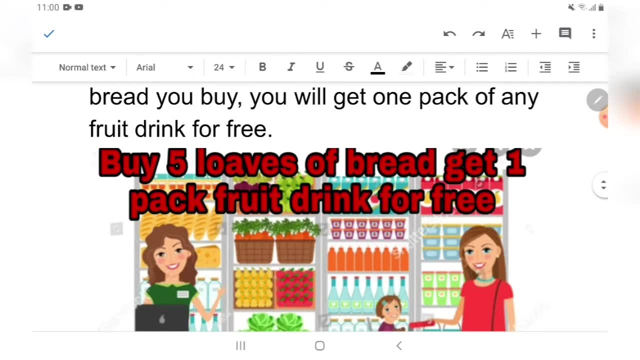 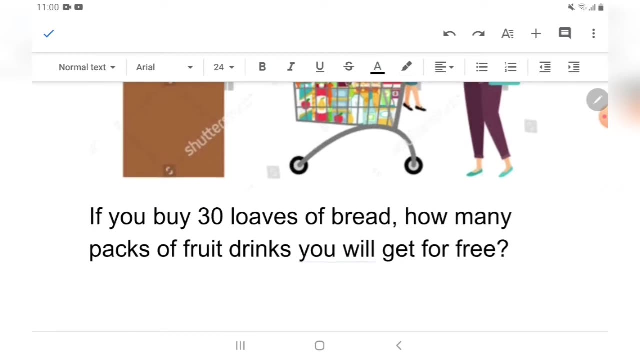 What is bread Bread? 5 loaves of bread you buy. Wait, You will get 1 pack of fruit drink for free. Wow, There is a promotion. So in here the problem here: If you buy 30 loaves of bread, 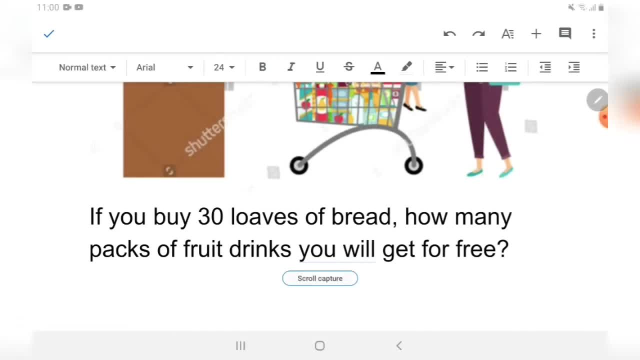 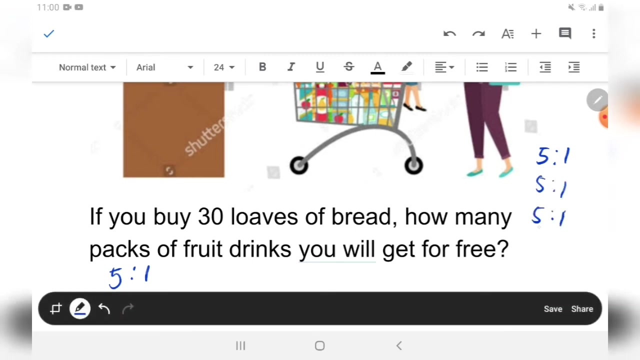 How many packs of fruit drinks you will get For free. So we know that if you buy 3, I mean 5- loaves of bread, you get 1 drink of 1 fruit drink. So in here, 5, 5, 5, 5, 10, 15,, 20,, 25,, 30. 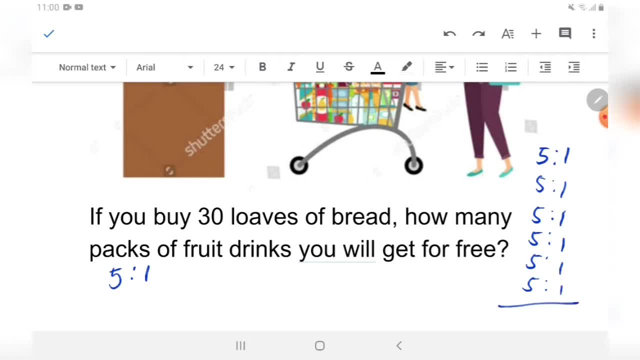 Okay, So how many fruit drinks you will get? That is 1,, 2,, 3,, 4,, 5,, 6.. And there are 6.. So we have here 30,, 2,, 6.. 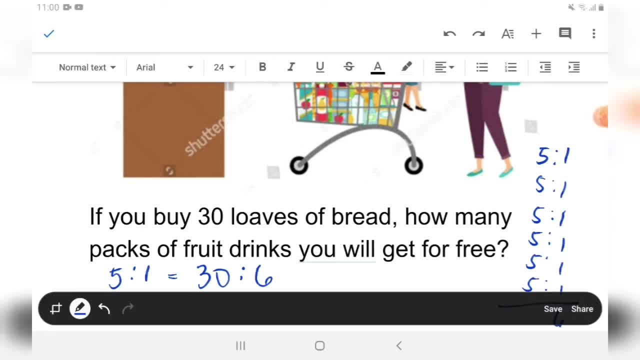 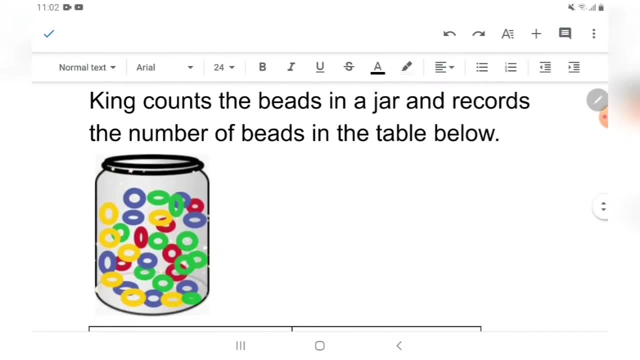 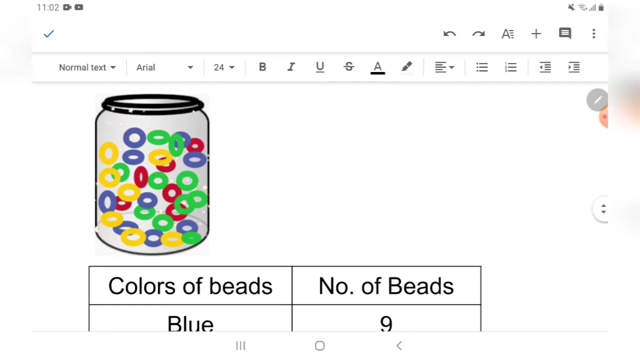 And that's it. We solved our problem that if you buy 30 loaves of bread, you will get 6 packs of fruit drinks for free. Very easy. Next, King counts the beads in a jar and records the number of beads in the table below. 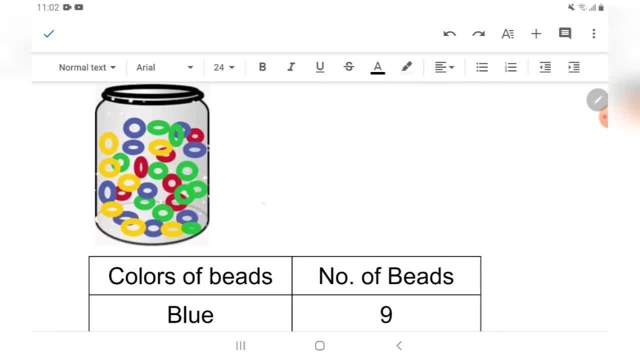 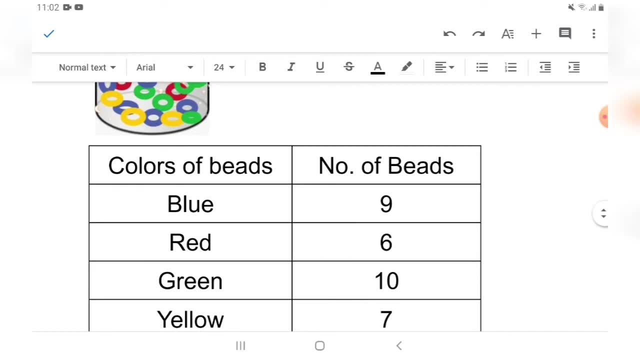 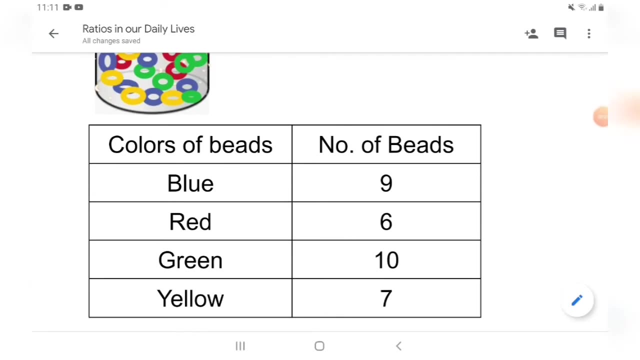 So in here this is the jar, and then inside of it there are beads. There are different colors of beads, And here the table shows that inside of the jar there are 9 loaves of bread. Okay, So there are 9 blue beads, 6 red beads, 10 green beads and 7 yellow beads. 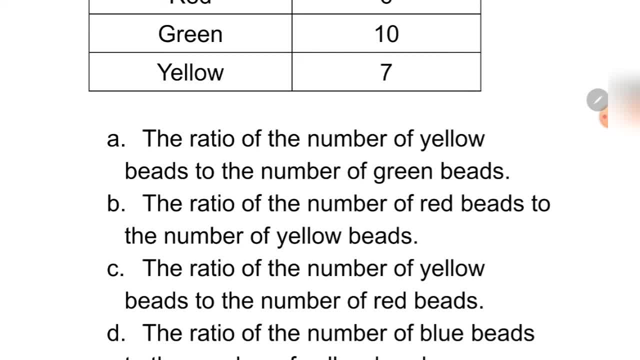 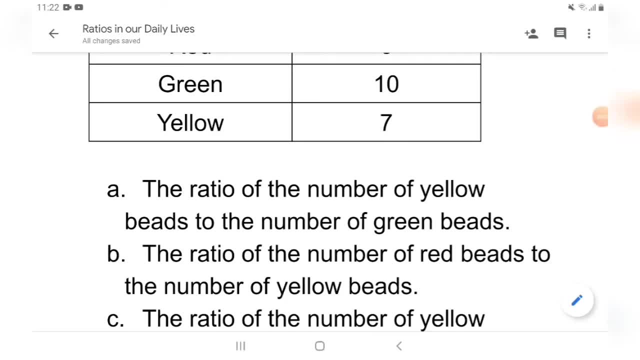 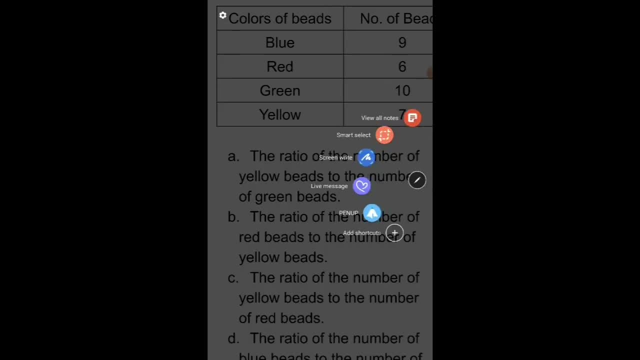 So the question are: what would be the ratio? or you're going to write the ratio of the number of yellow beads to the number of green beads. Okay, Let's make it smaller. Okay, Here Let's answer letter A: The ratio of the number of the yellow beads to the number of green beads. 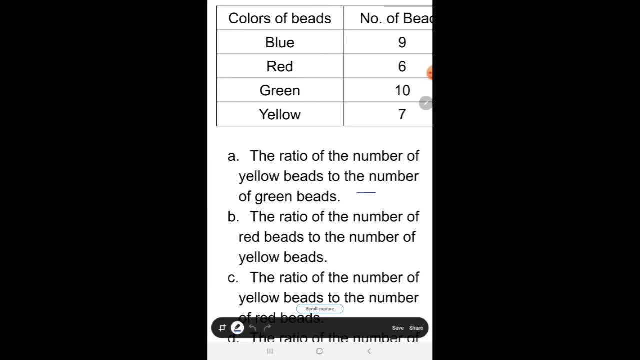 So how many yellow beads? That is 7 to green. That is 10 or 7 over 10.. Next, The ratio of the number of the red beads to the number of yellow beads. Red beads: That is 6 to yellow. 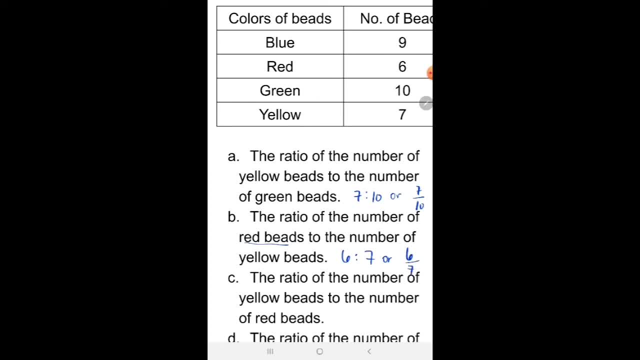 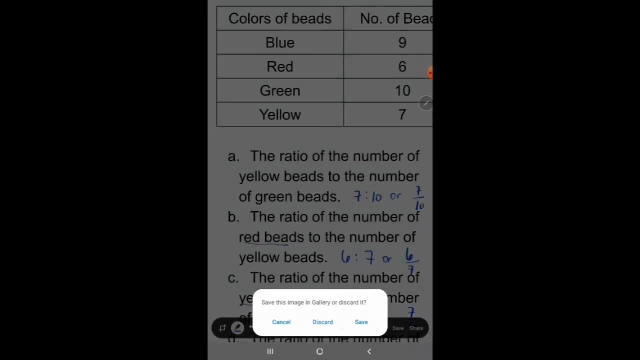 7 or 6 over 7. 7.. Next, The ratio of the number of yellow beads- Yellow 7 to red. How many? That is 6.. So 7 over 6. Very easy, right. Next, 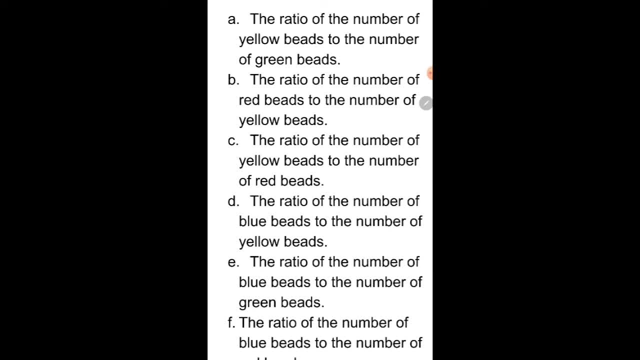 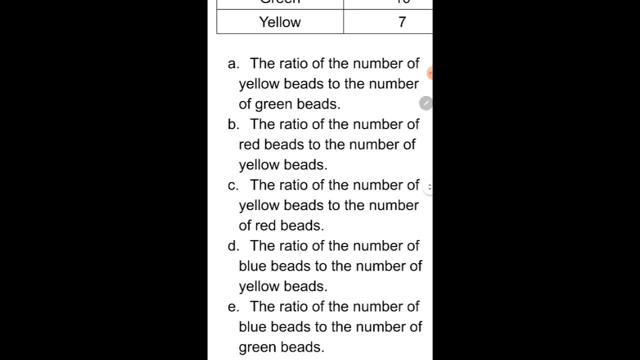 The ratio of the number of blue beads to the number of yellow beads. How many blue There are? 9. 9 to yellow, 7. 9 to 7.. Next E: The ratio of the number of the blue beads to the number of green beads. 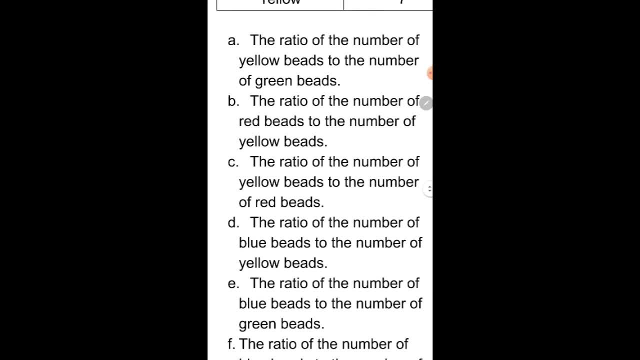 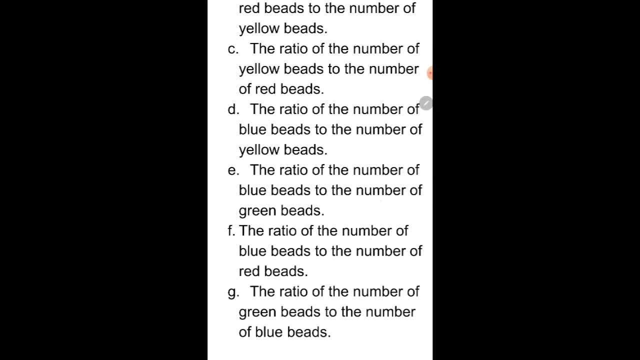 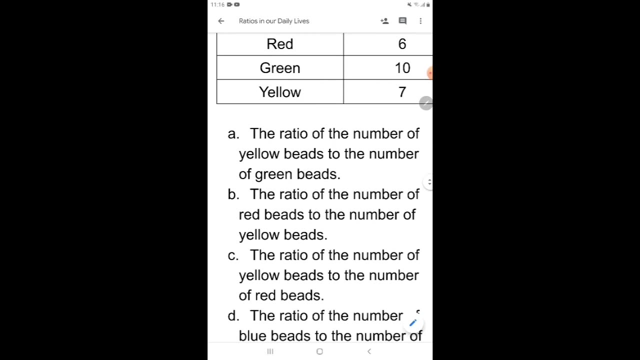 There are how many blue beads? 9 and then green is 10.. Next F, The ratio of the number of blue beads. There are 10 blue beads, 9 blue beads and then 10 green beads. Next The last. 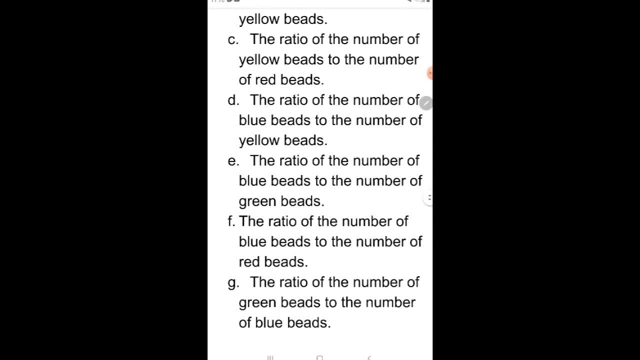 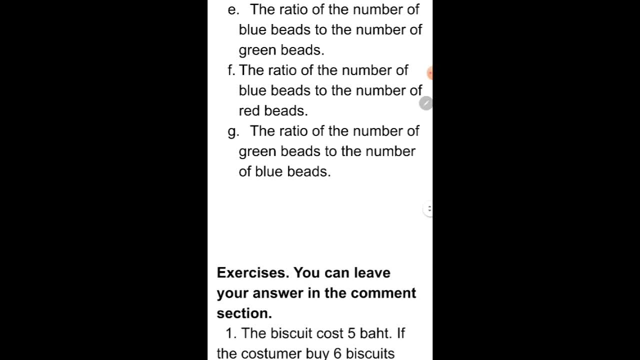 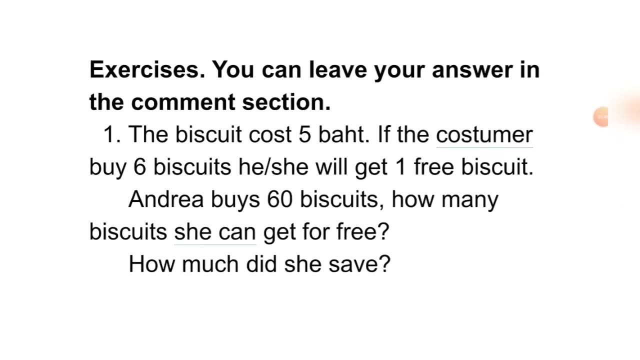 The ratio of the number of the green beads to the number of blue beads. There are 10 green beads and then 9 blue beads. So very easy. Next exercise: You can leave your answer in the comment section, Number 1 question. 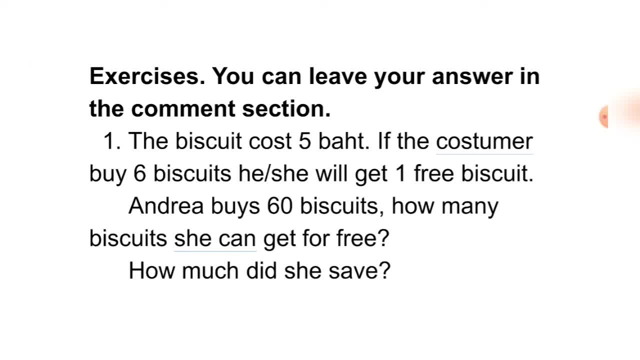 The biscuit costs 5 baht. If the customer buys 6 biscuits, he or she will get 1 free biscuit. Andrea buys 60 biscuits- How many biscuits she can get for free? And then next question is: how much did she save? 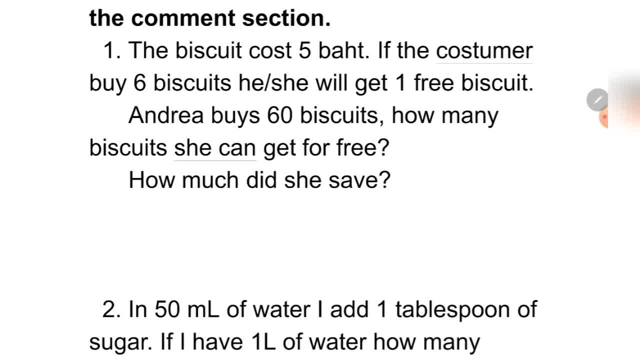 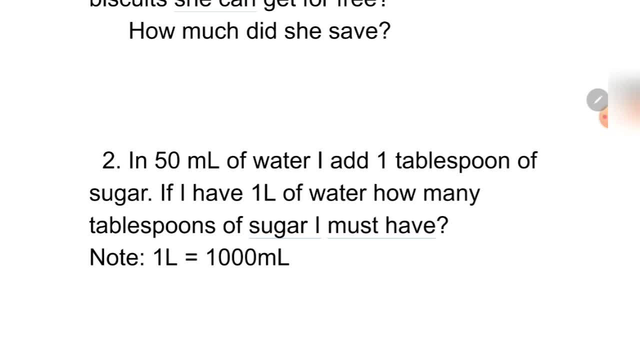 If you can't understand, you can use Google Translate. Next, number 2.. In 50 ml of water I add 1 tablespoon of sugar. If I have 1 liter of water, how many tablespoon of sugar I must have? 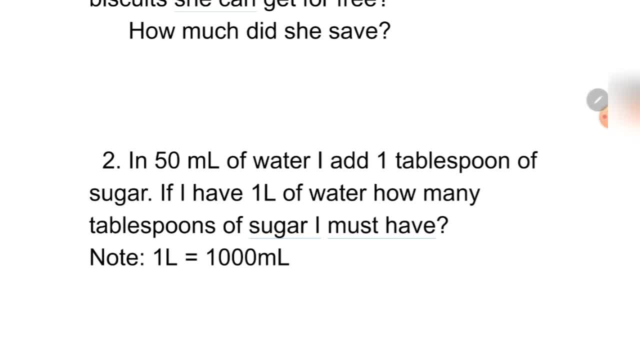 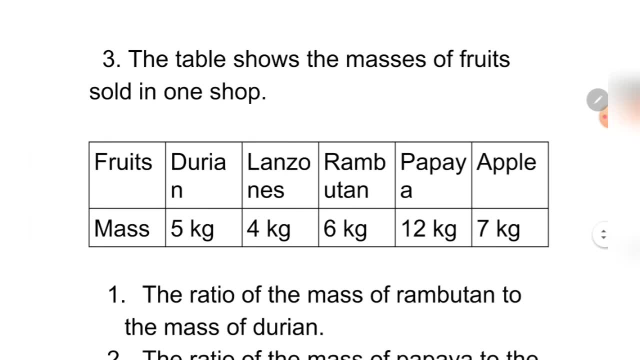 Note that in 1 liter there are 1000 ml Good luck Number 3.. The table shows the masses of fruits sold in one shop. This is the fruits: Durian Lanzones, Rambutan, Papaya. Apple. And then these are the masses: 5 kilogram of durian, 4 kilogram of lanzones, 6 kilogram of rambutan, 12 kilogram of papaya, 7. 7 kilogram of apple.